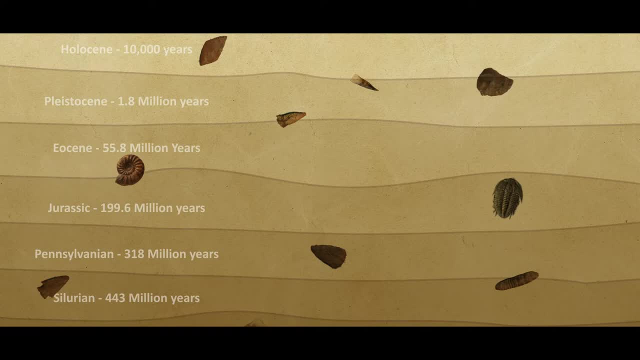 the oldest, as new layers are formed over it. We already have fossils belonging to each layer. Let us consider that we have discovered a new bone from the third layer, So by relating the bone to the shell of the same layer, we could presume that the bone and the shell belong to. 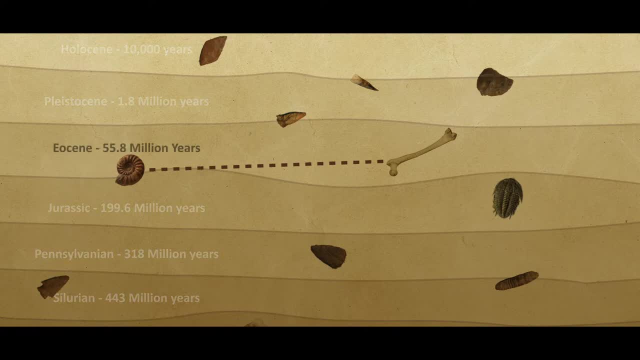 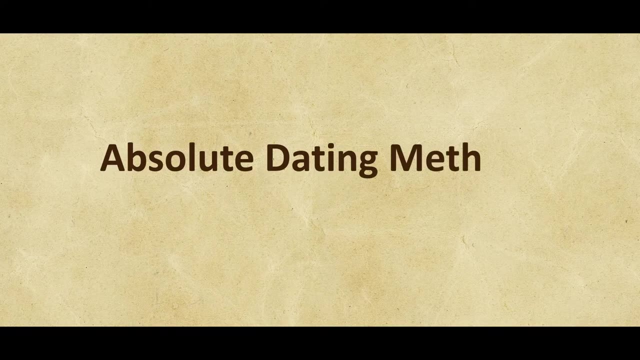 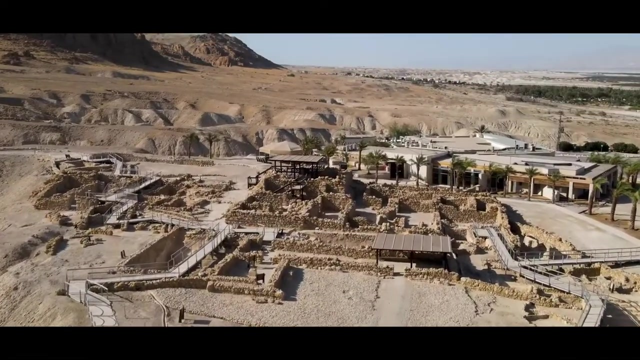 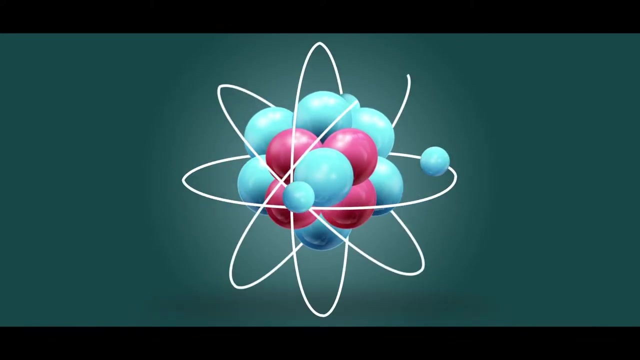 the same age. This method is called the Relative Dating Method. The other method is the Absolute Dating Method. Using this method, archaeologists are able to determine the numerical age of the fossil itself. We know that all elements are made of atoms. In order to understand this method, 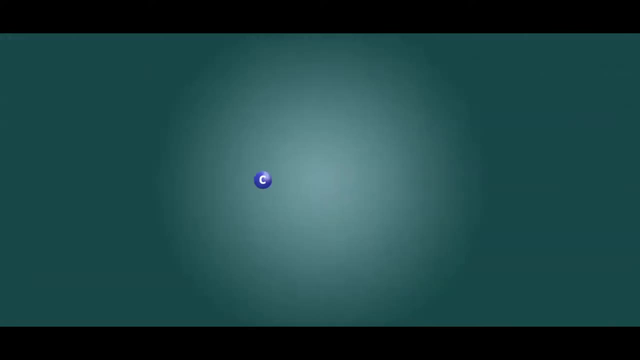 we need to go a little deeper into these atoms. Let us take the element carbon, for example. Carbon has six protons and six neutrons. This carbon is called carbon 12 or C12, which is a sum of protons and neutrons. The carbon atoms, which has six protons and seven neutrons, are: 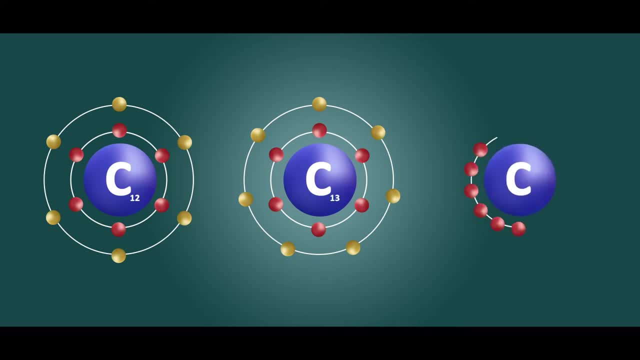 called carbon 13, and the ones with six protons and eight neutrons form carbon 14, C14.. So atoms with same number of protons and different number of neutrons are called isotopes of that element. Here C12, C13 and C14 are called the isotopes of carbon. 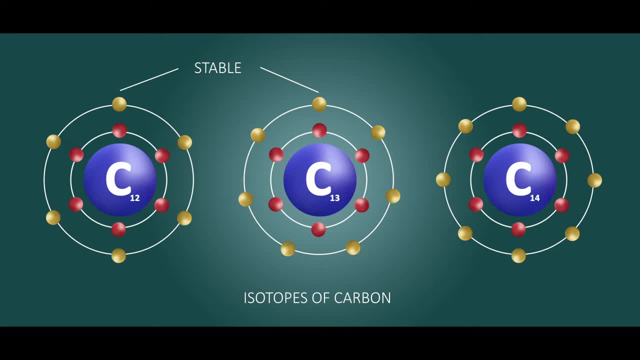 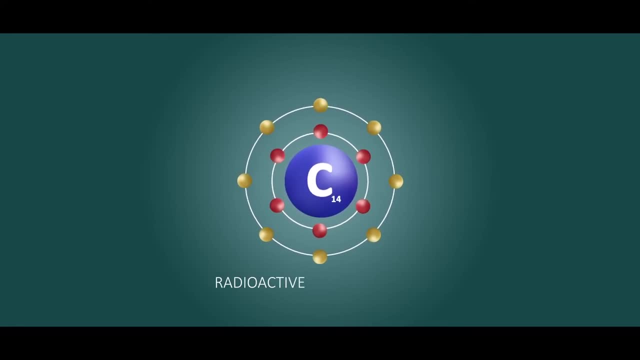 C12 and C13 are stable isotopes, but C14 is an unstable carbon. This unstable C14 is radioactive and when they decay, one neutron gets converted into a proton, which makes the number of protons and neutrons to seven, each making it a stable nitrogen atom. 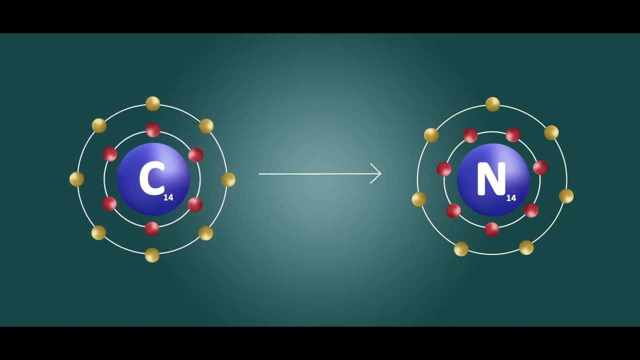 This process of carbon 14 becoming nitrogen 14 is called atomic decay. The time taken for this is 5730 years and this duration is called a half cycle. Why is this called a half cycle? Because when C14 decays to N14, only half the original sample of 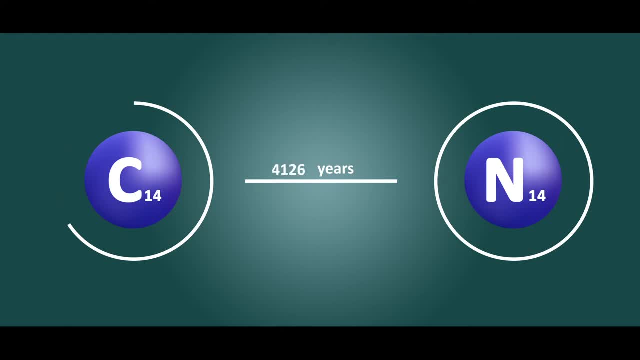 C14 remains in the organic matter. So after 5730 years only 50% of the C14 remains in the bone, And after each half cycle the amount of C14 keeps decreasing by 50% and around 70,000 years. 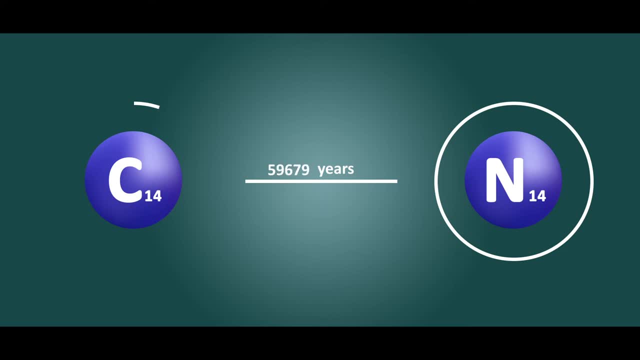 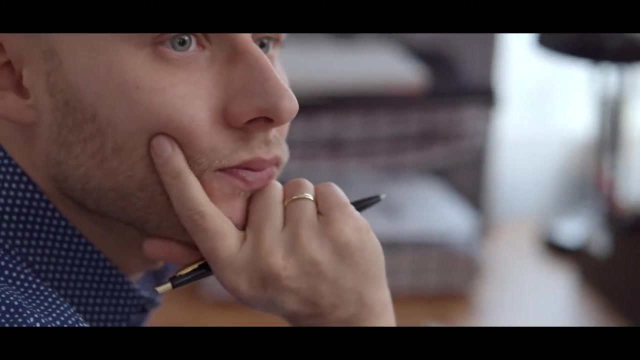 there is less than 1% of C14 left over, and it becomes very hard to detect C14 in the bone or any other organic matter, thus making it impossible to determine the age beyond 70,000 years. carbon for more than 50,000 years. how do we trace it back to millions of years? 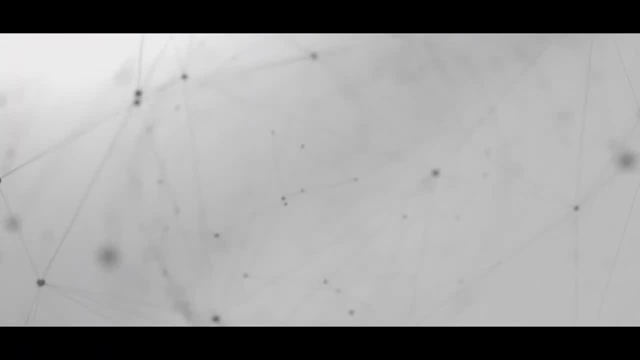 Well, every atom has unstable isotopes, just like carbon. The half-life of carbon is just 5730 years, but whereas half-life of potassium argon is 1.25 billion years, Using potassium argon dating we could determine the age range from 20,000 years to 4.5 billion years. But potassium 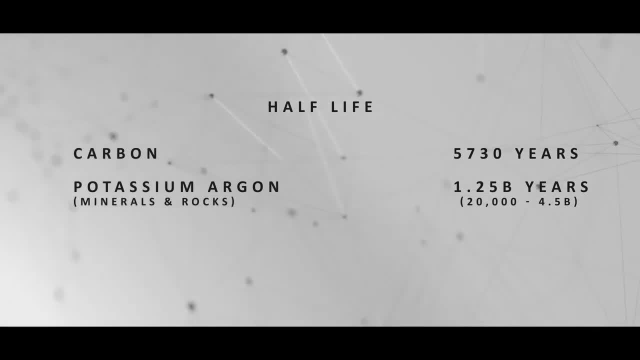 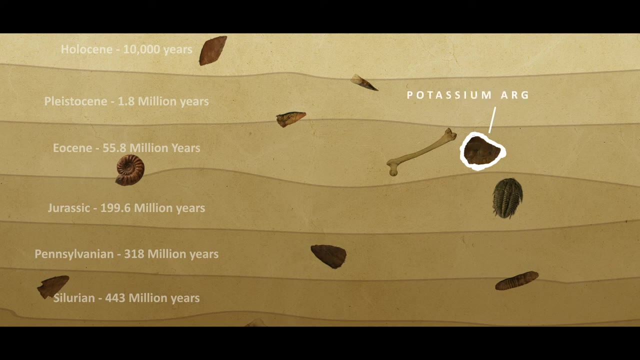 argon dating can be used only in minerals and rocks. How do we determine the age of bone using potassium argon dating? We take the help of relative dating method. If we could determine the age of the rock right next to the bone using potassium argon dating method? 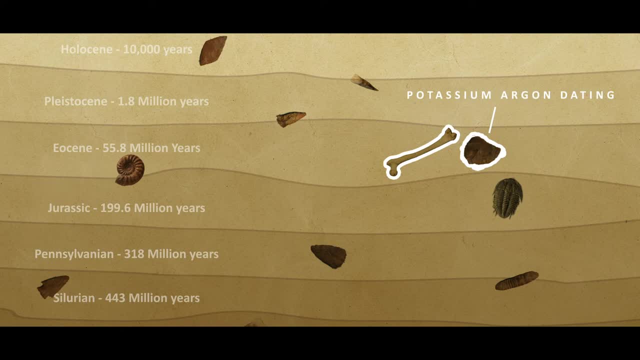 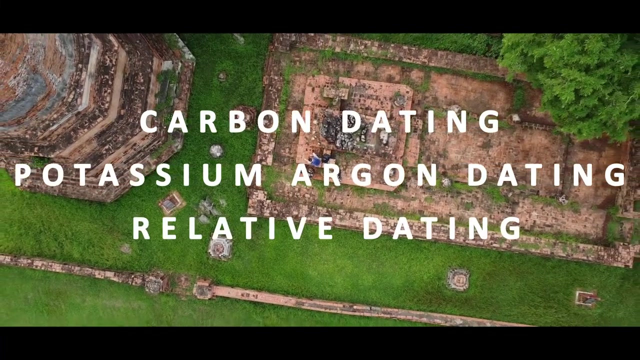 then we could determine the age of the dinosaur bones also belongs to the same strata, then we could presume that the rock and the bone belong to the same period. By combining various methods like carbon dating, potassium-argon dating and relative dating methods, archaeologists calculate the age of any fossil buried underground for over 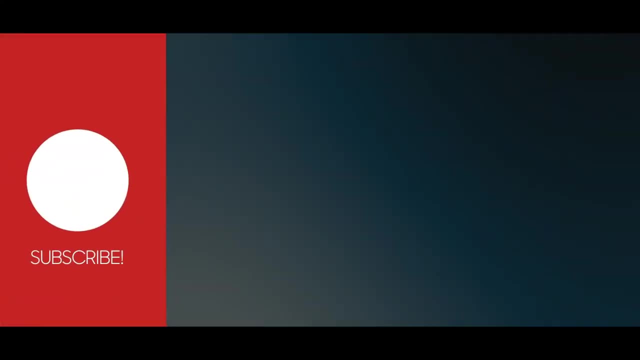 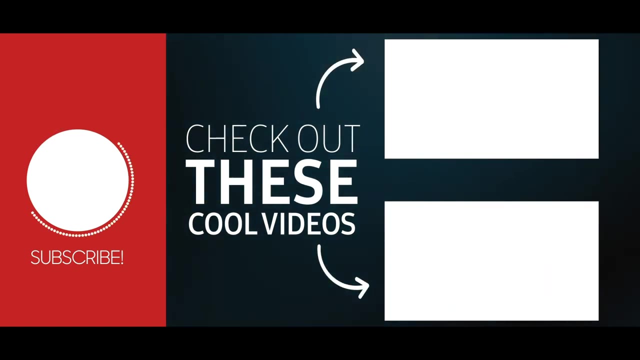 millions and millions of years. So that's it for this video. If you do like this video and our way of explaining things, give us a like, and if you have any such curious topic, let us know in the comments below. We will catch you guys soon with another interesting video like this. Until then, this is Team DNA. signing off bye, bye.